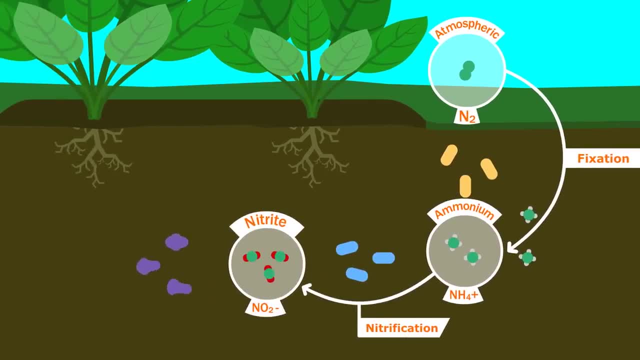 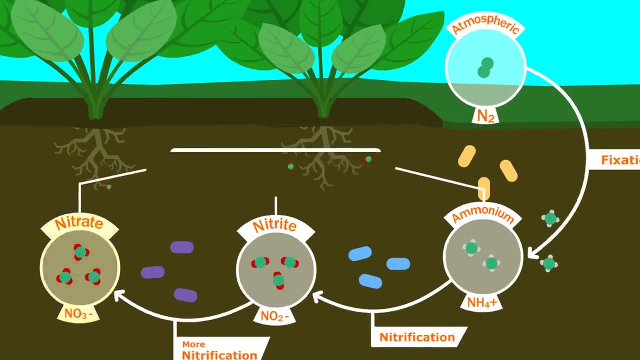 which poop out nitrite, which gets eaten by yet another kind of bacteria which poops out nitrate. All of these forms of nitrogen are available for plants, especially nitrate, which is the easiest for plants to use. Plants can take this up directly if it is near their roots. 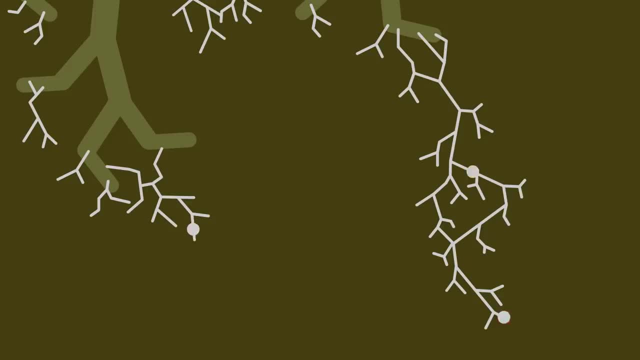 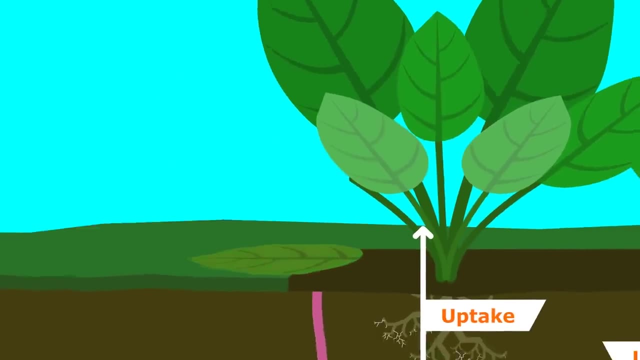 but they most often rely on strands of fungi that attach to their roots and bring nutrients to them in exchange for the sugars and carbohydrates the plant roots exude. Dead plant material is also rich in nitrogen and gets brought down with the help of worms, whose poop is a delicacy among nitrifying bacteria. Some of the ways nitrogen exits. 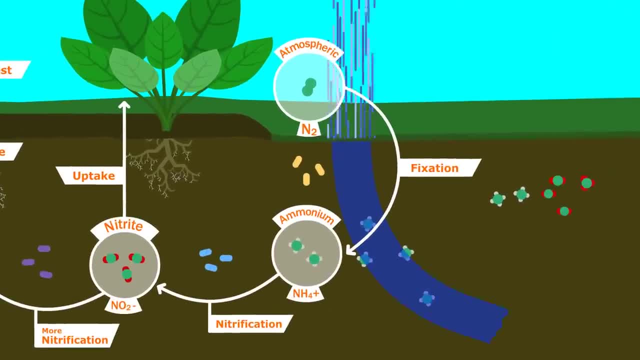 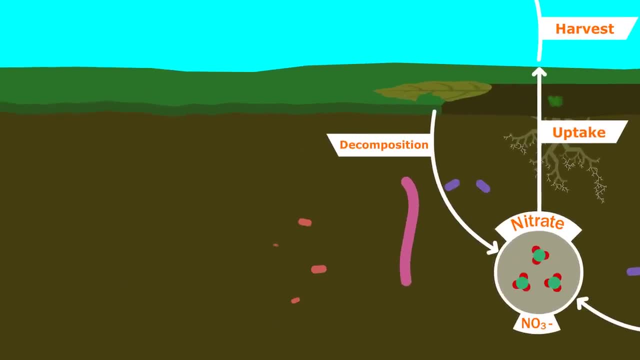 the soil is when the crop is harvested, when water carries it away, or when it becomes gaseous and returns to the atmosphere, Or if the soil lacks oxygen, different anaerobic bacteria grow which convert nitrates back into atmospheric nitrogen. Notice that these things only happen. 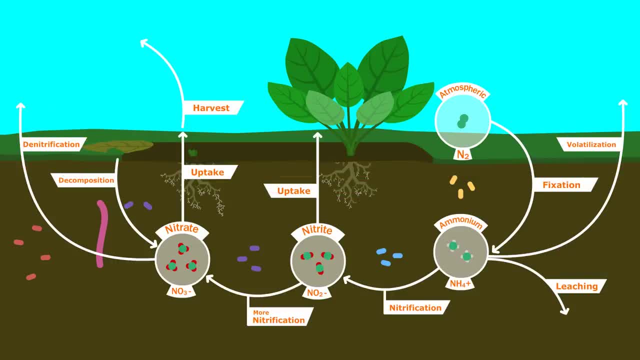 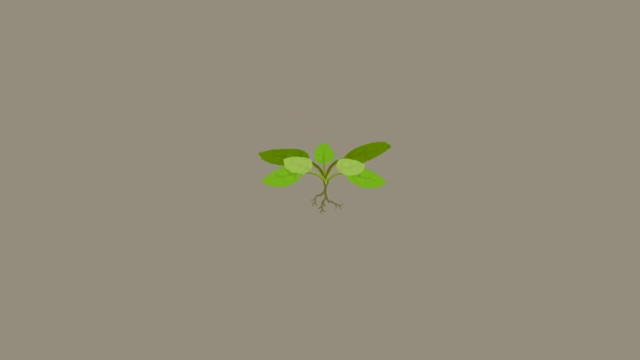 with loose nitrogen in the soil, not with nitrogen inside organisms. OK, so we know that the nitrogen cycle depends heavily on life in the soil. Without them, the plants would be quite sad. But you may have noticed if the fixation process is. 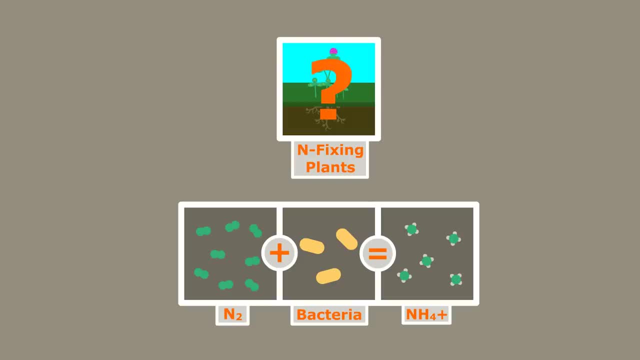 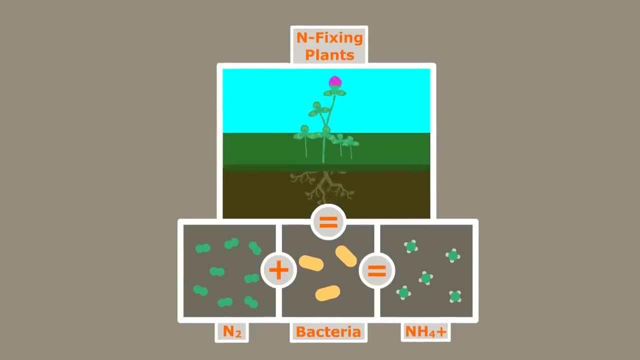 done by bacteria. where do nitrogen-fixing plants fit into this? Believe it or not, nitrogen-fixing plants don't fix nitrogen. Rather, they create habitat for the bacteria that do. The roots of this clover plant have little nodules that house huge amounts of nitrogen-fixing. 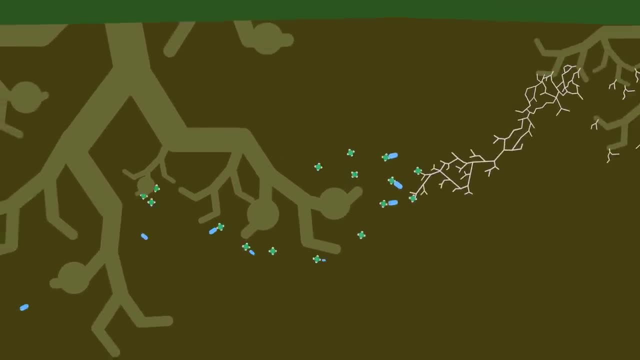 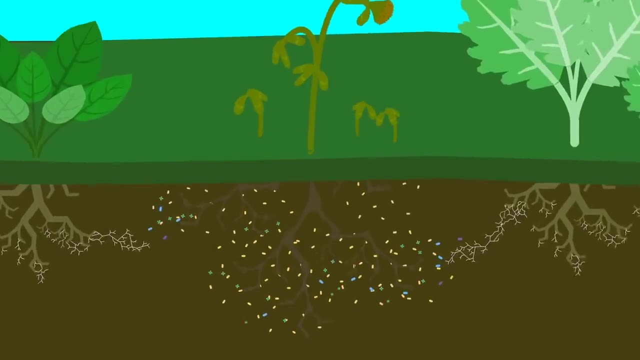 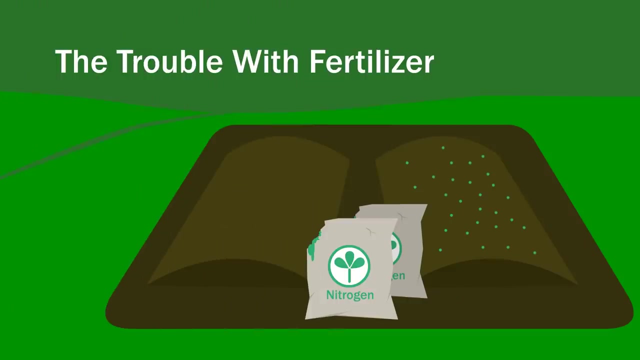 bacteria. The ammonium that these bacteria create slowly releases into the soil for neighboring plants and microorganisms to use. When the plant dies, the bacteria disperse into the soil, resulting in an abundance of bacterial allies for future plants' nitrogen needs. You know how earlier I said that water can carry soil nitrogen away. This nitrogen ends up in 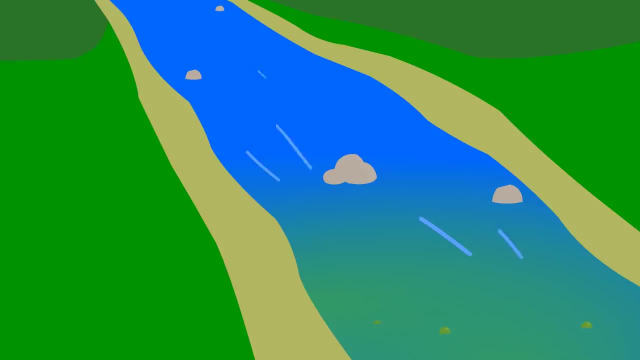 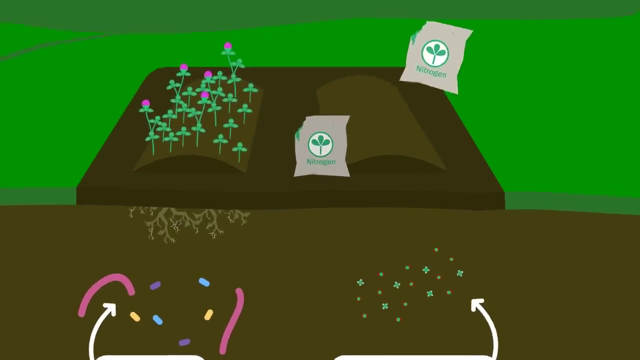 rivers, which can disrupt the ecosystem by enabling algae to dominate. But remember this only happens to loose nitrogen in the soil and not nitrogen embedded in organisms, And fertilizer adds pure nitrogen without the organism's presence. So nitrogen-fixing plants and microorganisms are. 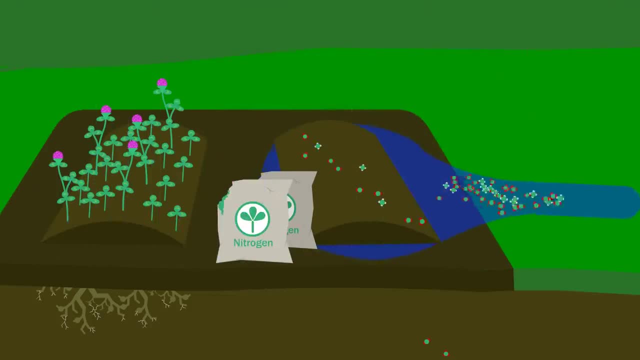 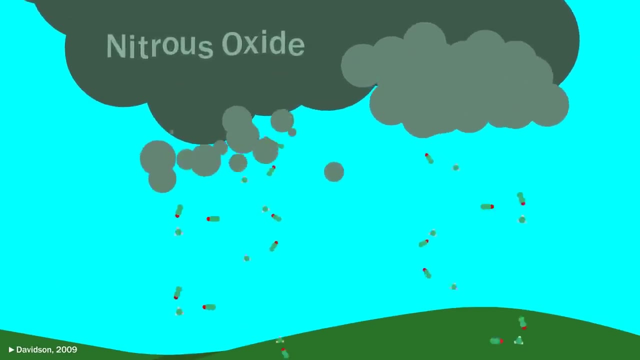 the only ones that can destroy the organisms. So when it rains, huge amounts of it run off and pollute the water. Loose nitrogen molecules are also much more prone to volatilization, releasing huge amounts of nitrous oxide, a potent greenhouse gas, into the atmosphere. 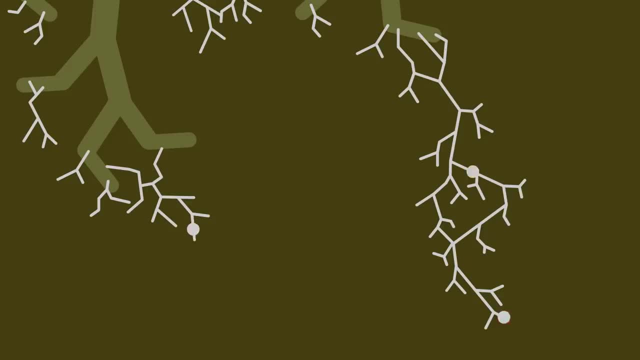 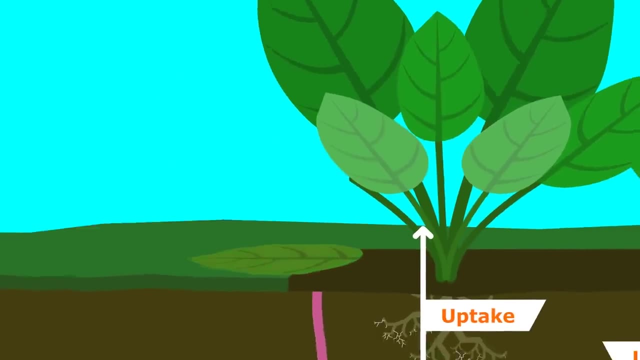 but they most often rely on strands of fungi that attach to their roots and bring nutrients to them in exchange for the sugars and carbohydrates the plant roots exude. Dead plant material is also rich in nitrogen and gets brought down with the help of worms, whose poop is a delicacy among nitrifying bacteria. Some of the ways nitrogen exits. 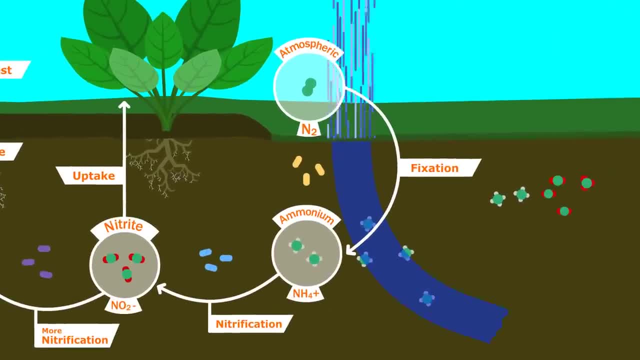 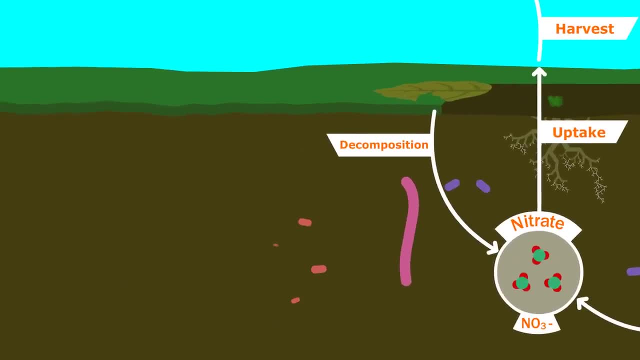 the soil is when the crop is harvested, when water carries it away, or when it becomes gaseous and returns to the atmosphere, Or if the soil lacks oxygen, different anaerobic bacteria grow which convert nitrates back into atmospheric nitrogen. Notice that these 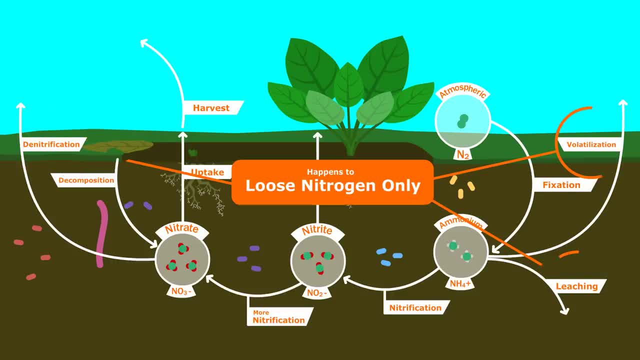 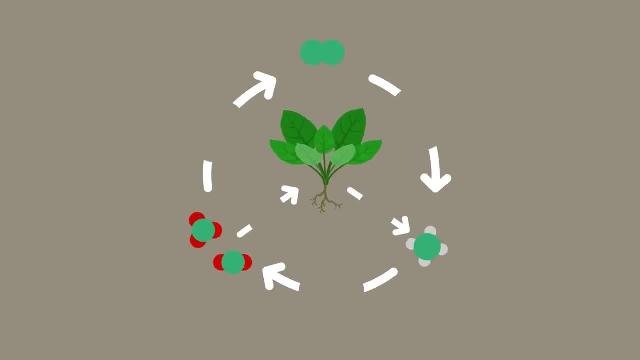 things only happen with loose nitrogen in the soil, not with nitrogen inside organisms. OK, so we know that the nitrogen cycle depends heavily on life in the soil. Without them, the plants would be quite sad. But you may have noticed, if the fixation process is done by 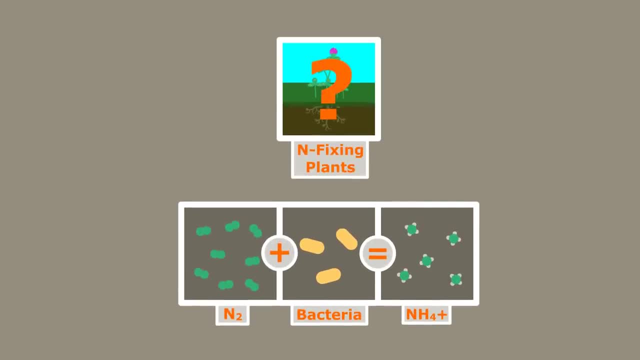 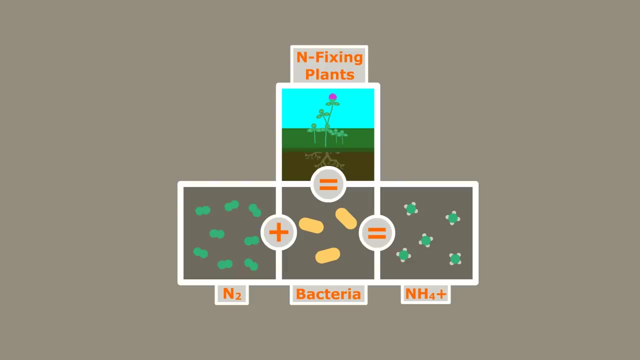 bacteria. where do nitrogen-fixing plants fit into this? Believe it or not, nitrogen-fixing plants don't fix nitrogen. Rather, they create habitat for the bacteria that do. The roots of this clover plant have little nodules that house huge amounts of nitrogen-fixing bacteria, The ammonium that 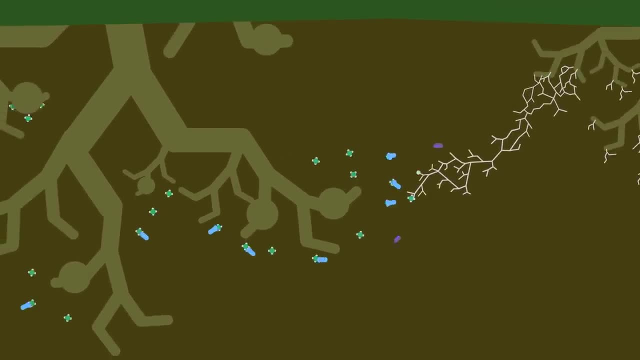 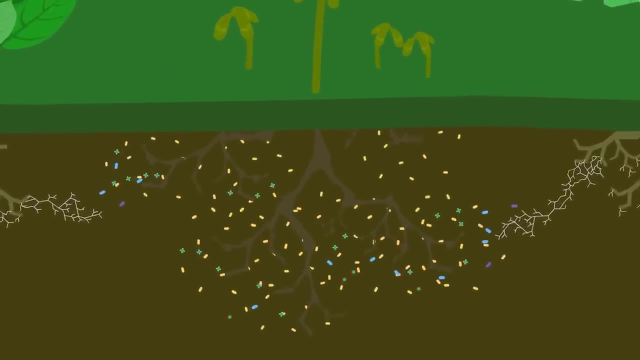 these bacteria create slowly releases into the soil for neighboring nutrients. The nitrogen-fixing plant has a lot of nitrogen in the soil, including the oxalic acid that is used as a nitrogen fertilizer. When the plant dies, the bacteria disperse into the soil. 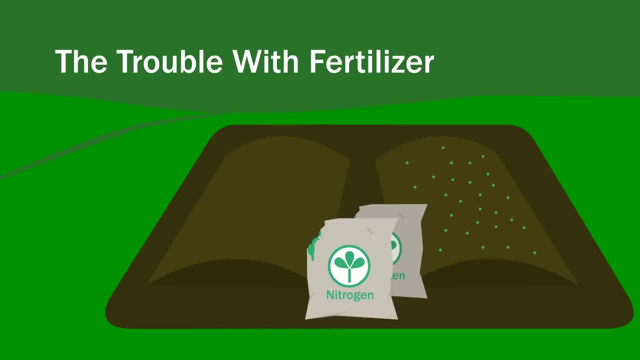 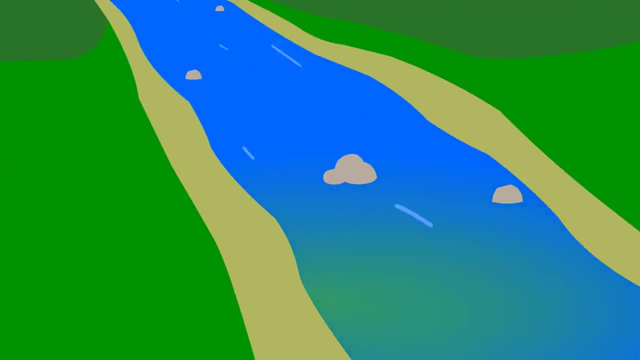 resulting in an abundance of bacterial allies for future plants' nitrogen needs. You know how earlier I said that water can carry soil nitrogen away. This nitrogen ends up in rivers, which can disrupt the ecosystem by enabling algae to dominate. But remember, this only happens. 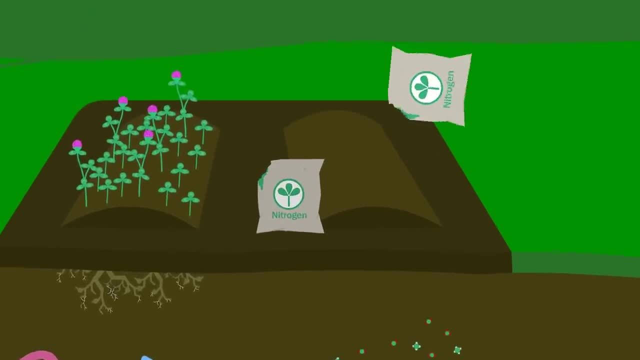 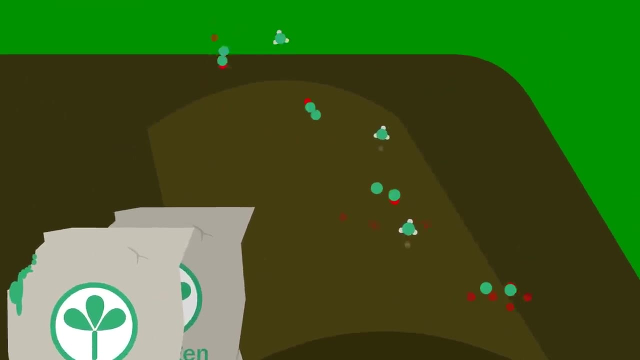 to loose nitrogen in the soil and not to nitrogen embedded in organisms And fertilizer adds pure without the organisms. So when it rains, huge amounts of it run off and pollute the water. Loose nitrogen molecules are also much more prone to volatilization, releasing huge amounts of nitrous oxide. 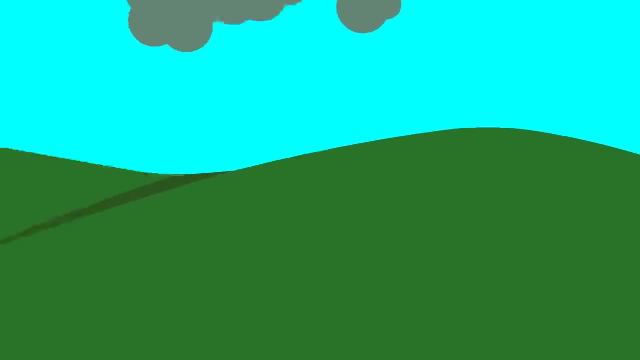 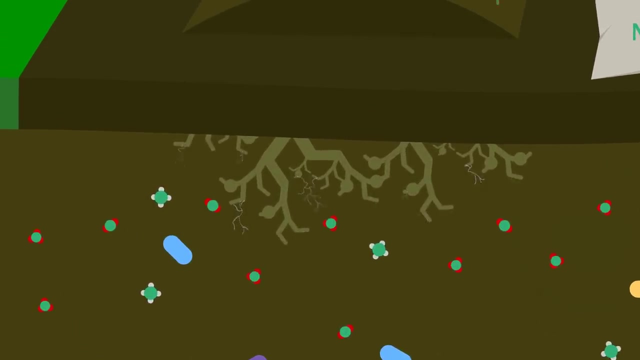 a potent greenhouse gas into the atmosphere. But that's not all. Such quantities of pure nitrogen irritate earthworms, which end up dying or leaving. It disrupts the helpful fungus on plant roots and changes the soil pH, making it inhospitable to bacteria.